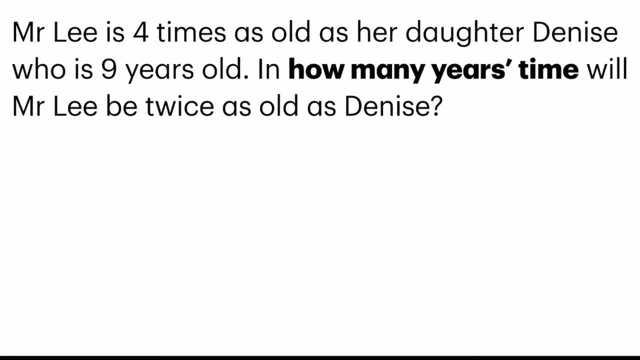 In age-related questions, it is helpful to know that the age difference between any two persons is always constant or the same. We call these the constant difference. For example, Mr Lee is 30 years old and Dennis is 5.. They have an age gap difference of 25.. This 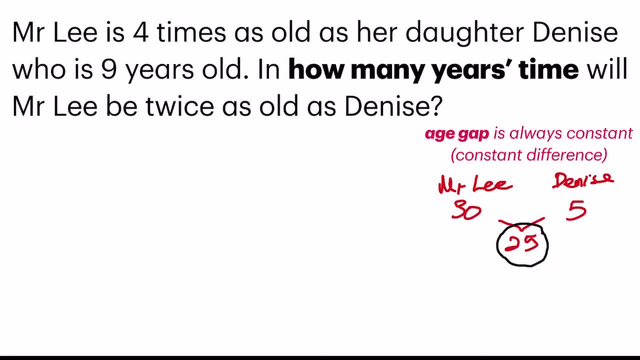 age gap difference of 25 is always the same every year. Why? Because Mr Lee will age by one year the year after and Dennis will also age by one year. So you see, since both of them increase in age of plus 1 and plus 1, the age gap difference is constant. So 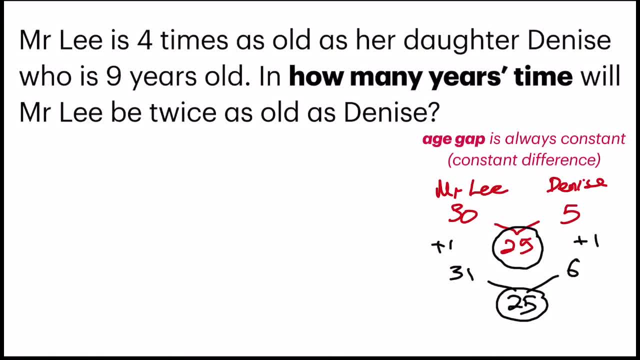 now let's tackle this question. Mr Lee is 4 times as old as his daughter, who is 9 years old. In how many years' time will Mr Lee be twice as old as Dennis? So remember just now what we have mentioned. 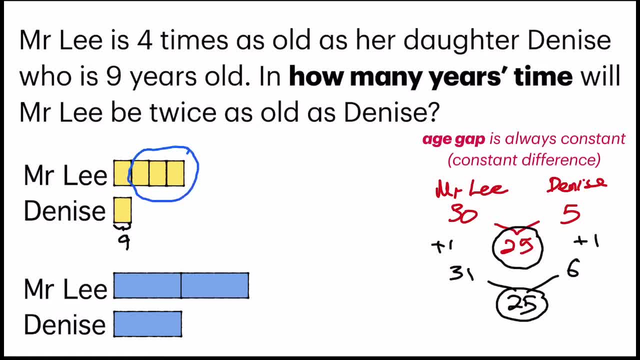 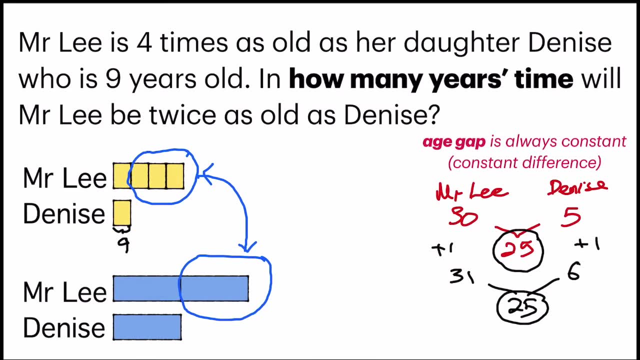 the age gap difference is always constant, So let us highlight the difference here, which means that these three units would be the same as this one chunk of blue unit. So let us find out what is the age gap. So in the first part it's 9 times 3.. I get 27,, which is equal to these three units. 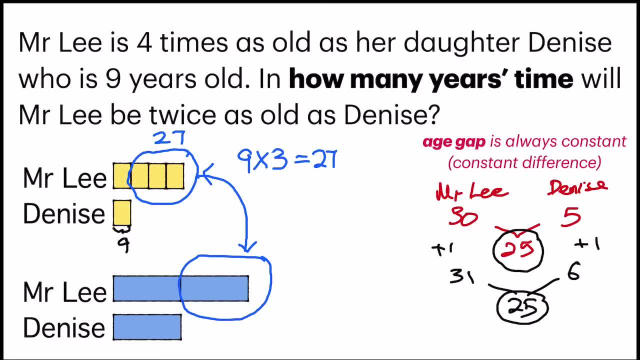 of yellow blocks, And then these three units of yellow blocks is equal to this one unit of blue block, which is Mr Lee's and Dennis' age gap, So which means this is 27, and Dennis would be 27 years old as well. 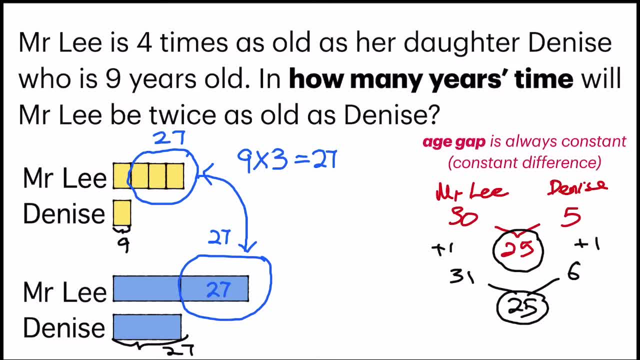 Okay, So what does this mean? So in the first part it is 20 times equal to 10, which means Dennis is 27 and Dennis was 8 years old. So let's deal with this question. So please show one example. 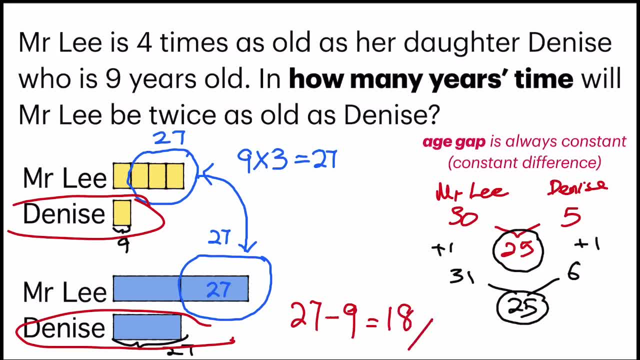 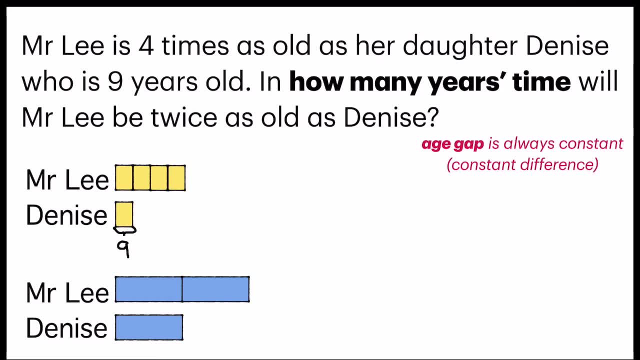 Will Mr Lee, when he was 17 years old, be twice as old? So in the first part it was: how many years' time about will Mr Lee be twice as old? We will look at Dennis' age. Dennis was 9..